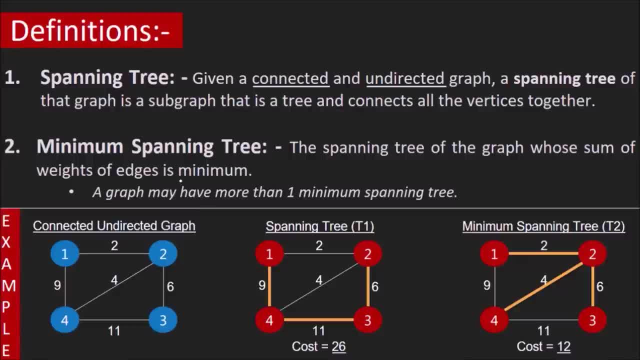 number of spanning trees, but not all of them are minimum. A minimum spanning tree is one in which the sum of weight of edges is minimum. For example, consider the given graph shown here. The edges highlighted in yellow are the edges of the spanning tree. Now, both the 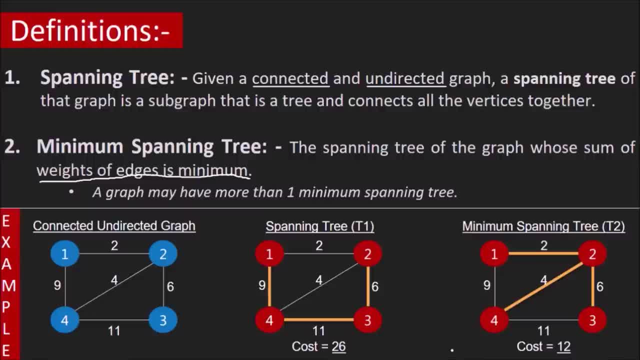 trees shown here form a spanning tree because each of these contain 4 vertices, are connected and do not contain any cycles. But tree 2 here has a cost lower than tree T1.. In fact tree 2 is a minimum spanning tree, so the sum of weight of its edges would be lower. 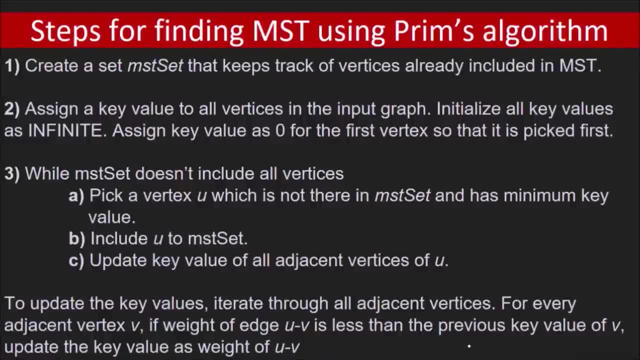 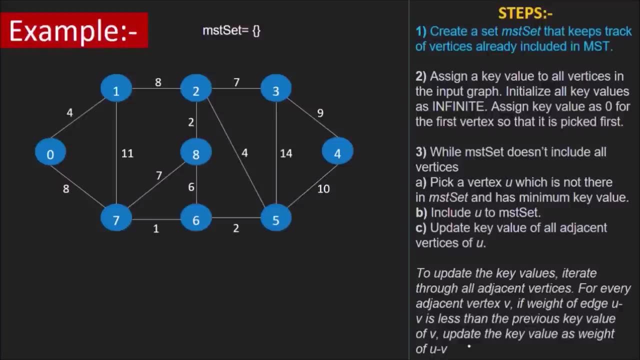 than any other possible spanning tree of a graph. Steps for finding a minimum spanning tree using Prim's algorithm. Well, it would be better if we try and understand each step one by one with the help of an example. So let's do that. Consider the given graph, which has 9 vertices, V0 to V8.. The numbers on the 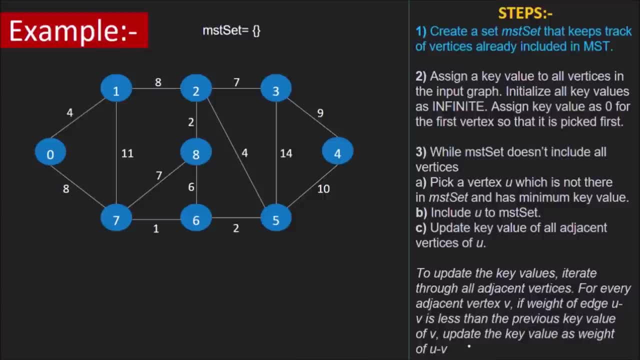 edges represent the weight of that edge. We need to obtain a minimum spanning tree of the given graph. The first step says: create a MST set which contains all the vertices in the minimum spanning tree. Initially this set will be empty, of course. Let's look at step 2.. It says that initialize the key of all vertices except the source. 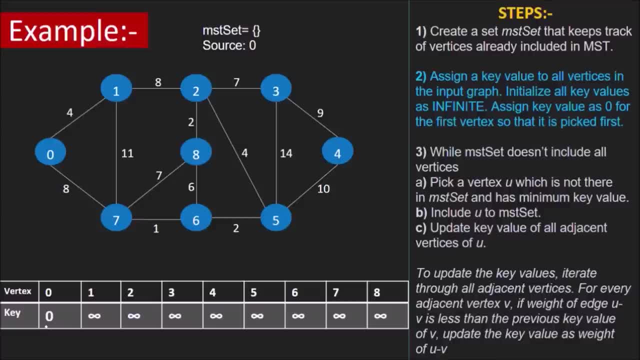 vertex to infinity. The source vertex is assigned key 0. Basically, the key of every vertex stores the weight of the minimum weighted edge it is connected to such that the other endpoint of that edge is a vertex in MST set. It will be clearer as we proceed through the 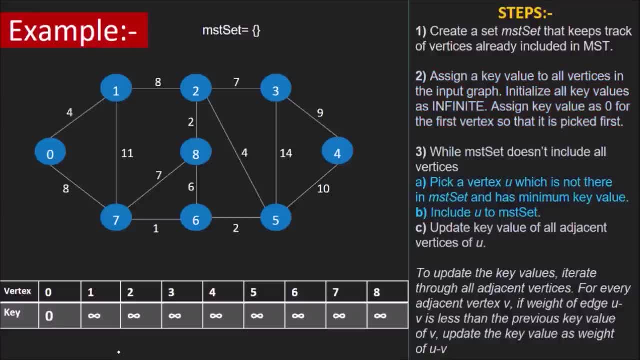 example. Now we need to pick a vertex U, not in MST set, with minimum key value. Since no vertex is in MST set initially, we need to look at all the vertices Here. V0 has a key 0, while all other vertices have key infinite. So V0 has the minimum key and hence it will be added. 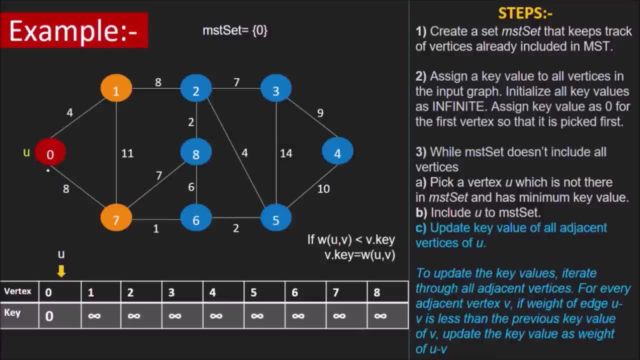 to our MST set. Now here, the vertices in red represent those vertices that are added to the MST set, while those in orange represent all the vertices adjacent to our current key vertex u, which are not in MSTZ. According to the next step, we need to update the key. 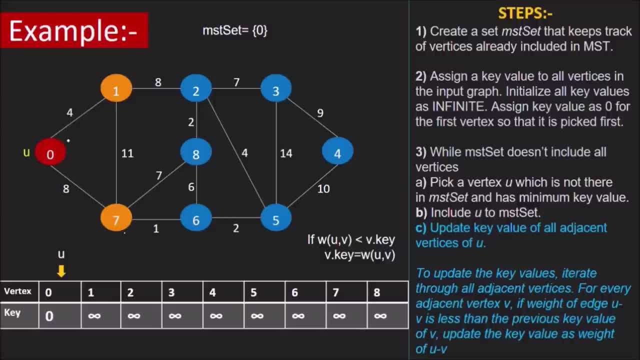 values of all vertices adjacent to u, which are v1 and v7 in this case. Now how to update the key values. It's simple. If the weight of edge uv is less than the key of v, update the key value as weight of uv. We see that weight of edge 0,1 is 4, while the key of 1. 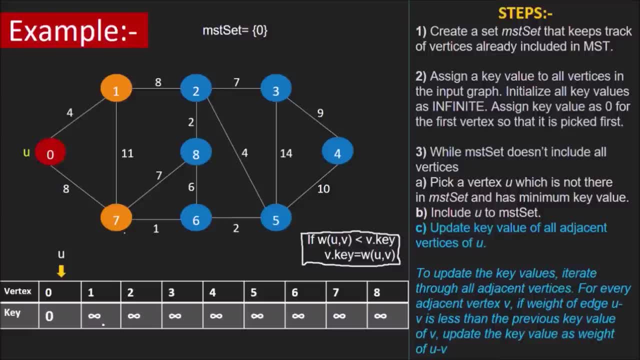 is still infinite. So we will update the key of v1 to 4.. Similarly, the weight of edge 0,7, which is 8, is less than key of 7, which is again infinite. It implies we need to update the key of v7 to 8.. Again, pick the vertex with minimum key, not in MSTZ, which is v1 in. 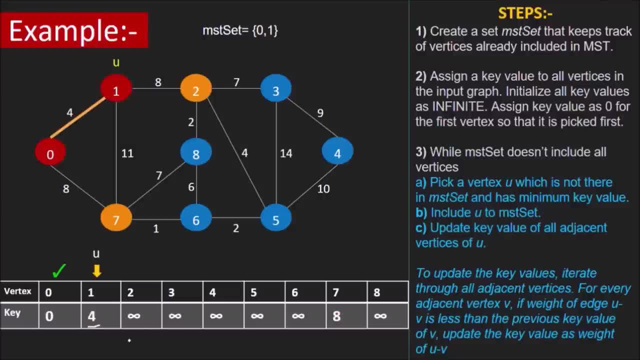 this case with key 4.. Add it to the MSTZ Here: v2 and v7 are the vertices adjacent to u. Now let's come to the next step. We need to update the key values of all vertices adjacent to u, which are v1 and v7 in this case. Now how to update the key values of all vertices. 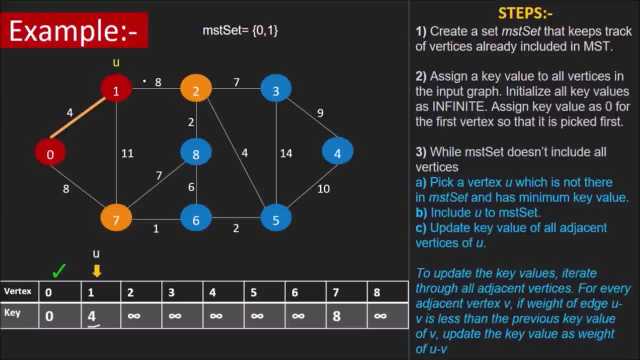 Now we again see that the weight of H12, which is 8, is less than the current key of V2.. So key of V2 will be updated to 8.. But on the other hand, weight of H17 is 11, whereas the key of V7 is already 8.. 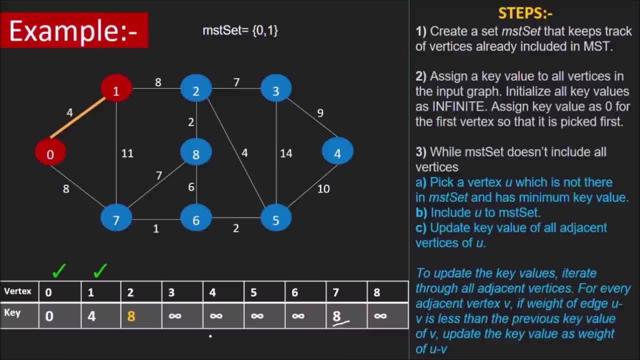 So the key of V7 won't be updated Again. pick vertex with minimum key, not in MST set. Both V2 and V7 have lowest keys so you can add either to MST set. Let's add V7.. V8 and V6 are adjacent vertices of V7, not in MST set. 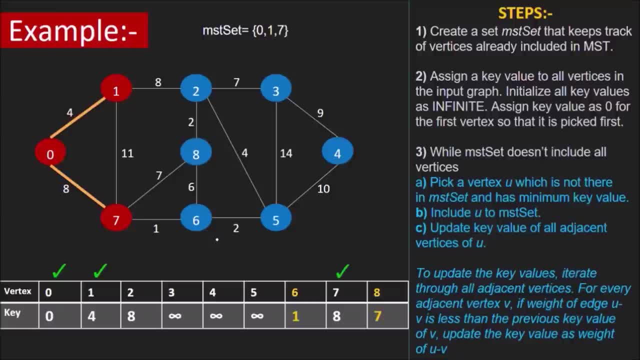 We'll update their keys following the same procedure as earlier. Next vertex to pick is V6, which has the lowest key of 1.. V8 and V5 are the vertices adjacent to our U ie V6. Weights of both V6, V5 and V6, V8 are less than the keys of V5 and V8 respectively. 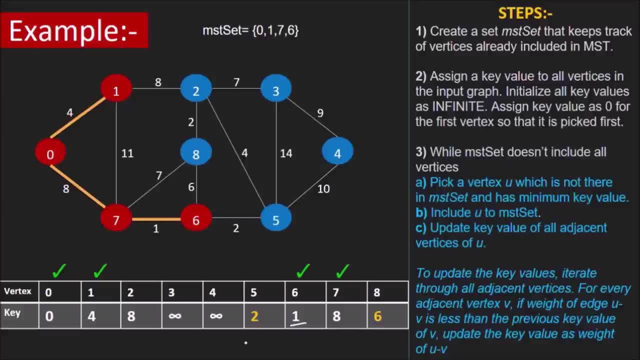 Update their keys too. Now let's see how we can change the key of V7.. V5 will be picked because it has the lowest key too, among all the vertices not in MST set. Now V5 has 3 adjacent vertices not in MST set, namely V2, V3 and V4.. 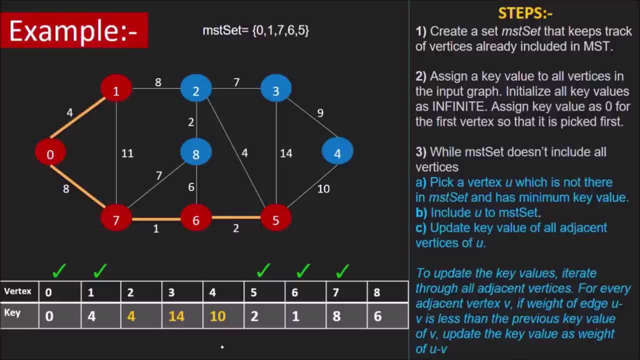 Keys of all the 3 will be updated. Among the 4 vertices not in MST set, V2 has the lowest key. With V2 as U, we find its neighbouring vertices not in MST set- V3 and V8- and update their keys following the same rule as earlier. 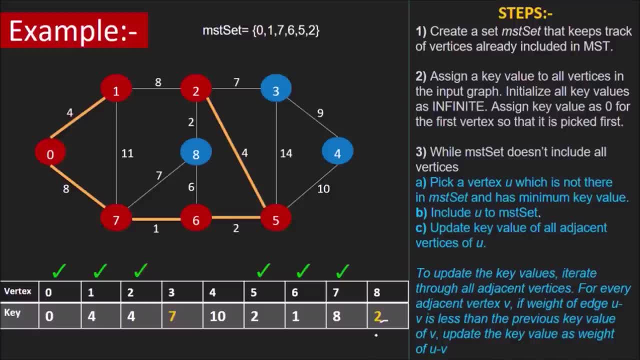 Now V7 has the lowest key 2, which is when we want to update my data centre. The keys are less than and not in MST set V2.. I'll update it before I pick V8 and V7, since V8 have the lowest key 2 added to the MST. 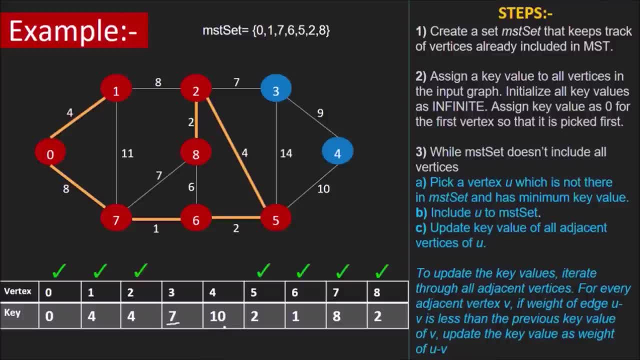 set. Now V8 has the lowest key. 2 added to the MST set V7.. V8 has no vertex adjacent to it, not already a part of MST set. Thus no keys will be updated in this case And V3 will be picked now because its key is less than that of V4, which is the only. 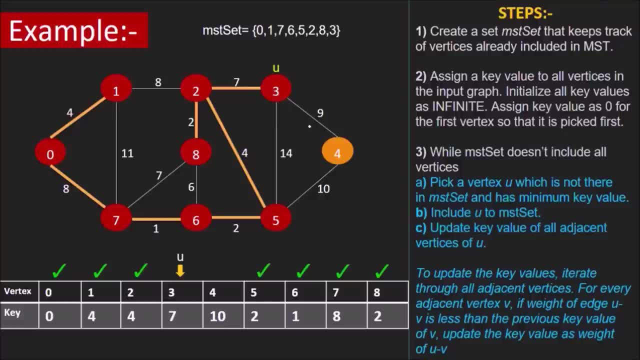 other vertex left not in MST set To update the keys. consider the only adjacent vertex of V3, which is V4.. Its weight is less than the current key of V4, which was 10.. It will executeutter v3 after this. 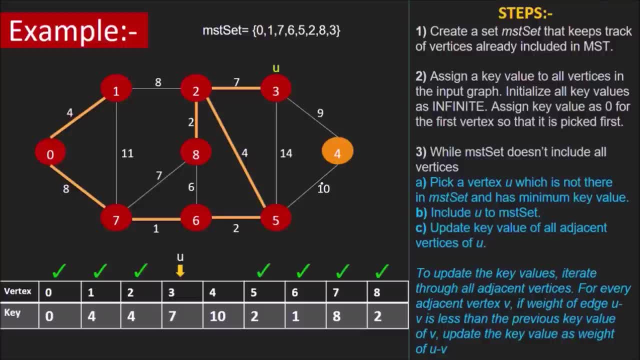 is v4. Its weight is less than the current key of v4, which was 10.. So set v4's key to 9.. Pick the last remaining vertex, v4, and add it to the MST set. Note that our condition says that the procedure will continue till all the vertices are not part of the MST set. 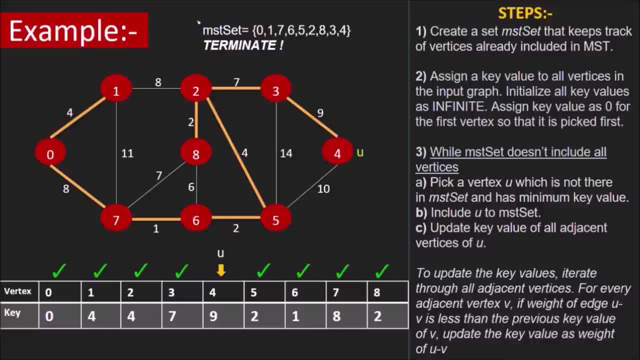 Since all the vertices are now added to the MST set, we have reached the terminating condition. Thus we have successfully obtained the minimum spanning tree of the given graph. We can also calculate the weight of the minimum spanning tree by adding the weight of individual edges. 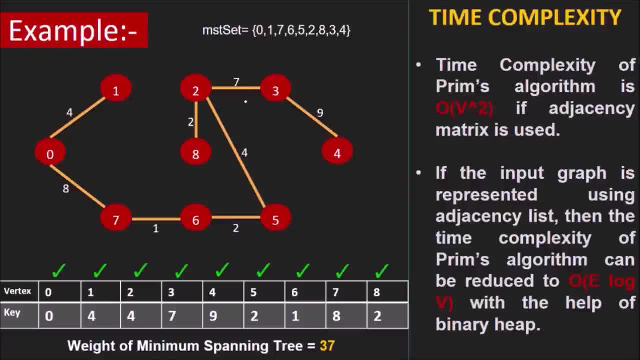 in this tree We see that they add up to 37. Now let's analyze the time complexity of Prem's algorithm. Now the time complexity of Prem's algorithm is O if implemented using adjacency matrix and O if done using adjacency list and binary. 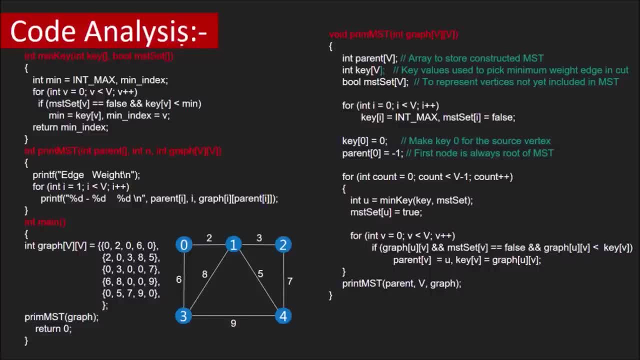 here. Now let's analyze the code for Prem's algorithm. This is an adjacency matrix implementation of the algorithm. Let's start with the main function. We've initialized the graph with the following matrix: The graph contains 5 vertices, 0 to 4.. Here, 2 represents there's 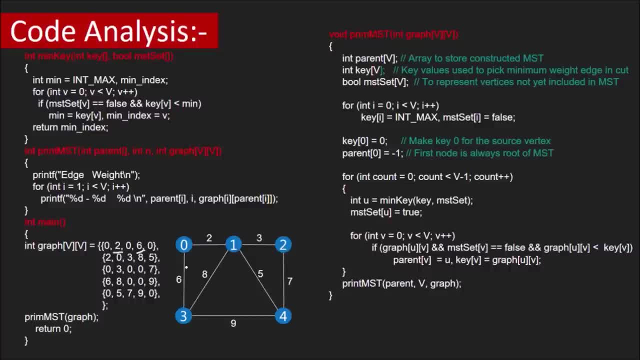 an edge between vertex 0 and 1 with weight 2 and 6 represents an edge between vertex 0 and 3 with weight 6 and so on. Now we call this function Parent error stores are constructed, MST key stores, the.